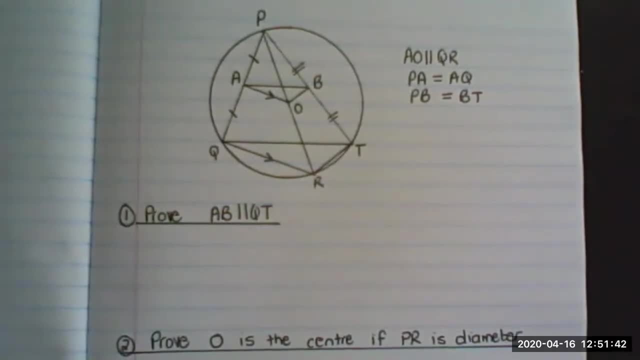 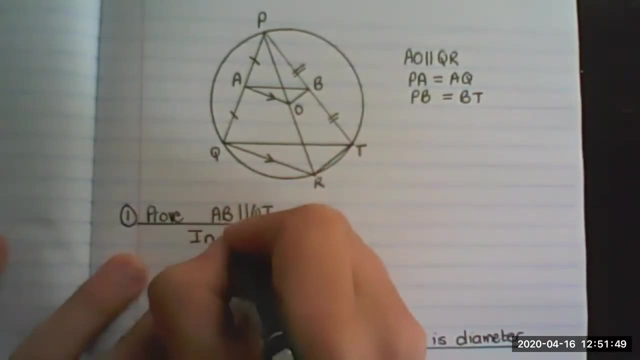 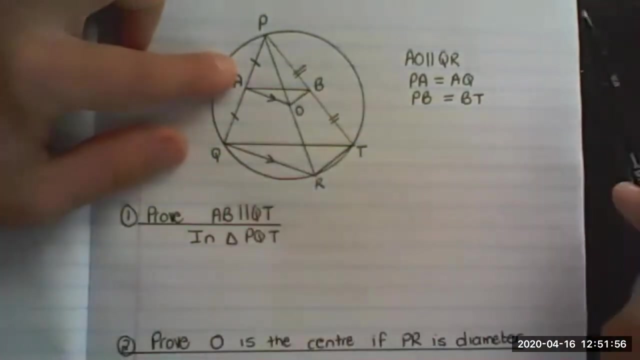 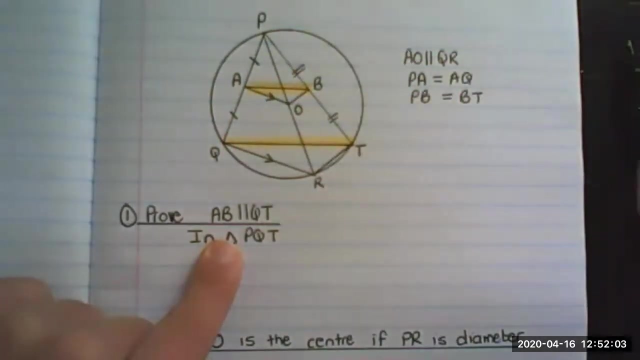 Okay, So prove: AB is parallel to QT And the way we solve it, as we say in triangle PQT. now look carefully what is happening. AB is this line and QT is that line. all right, And it forms part of this triangle. 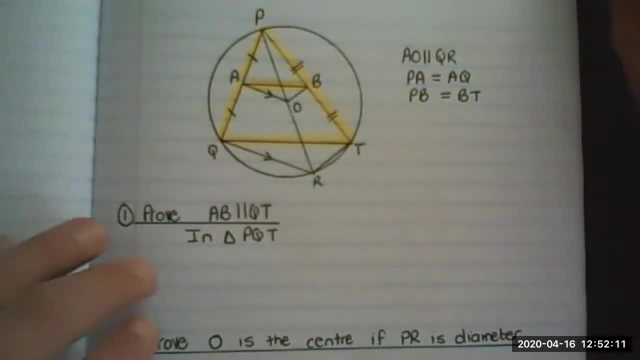 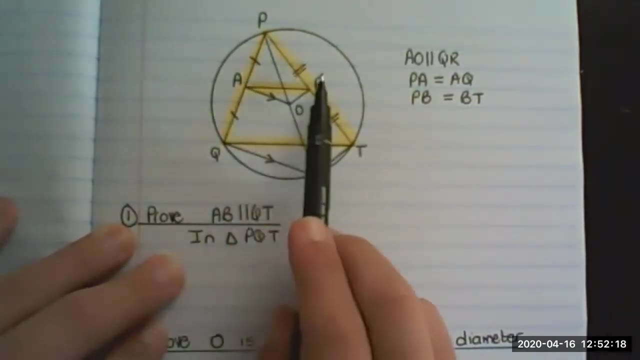 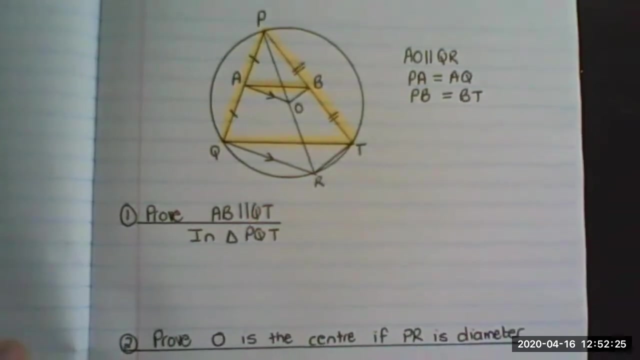 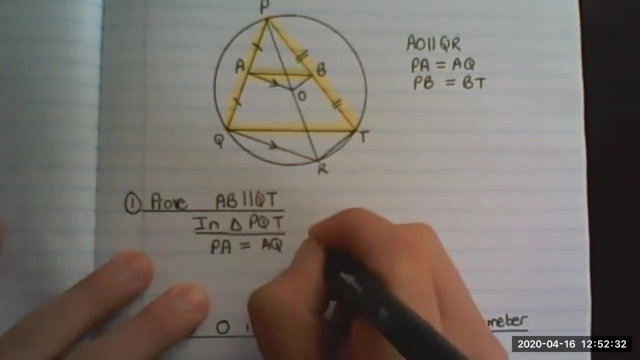 Okay, So now that it's part of this triangle, I can see that these pairs of lines are equal to each other. Therefore, this line is parallel to that one. So we say PA is equals to AQ and PB is equals to BT. 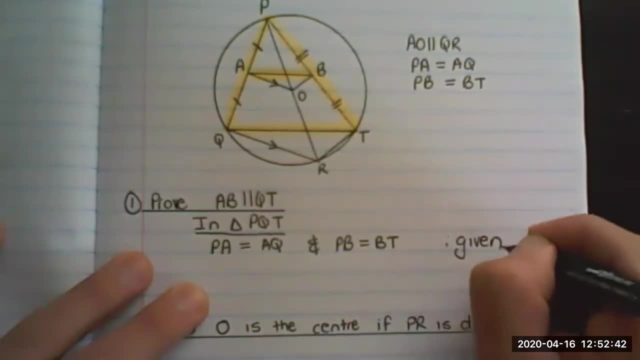 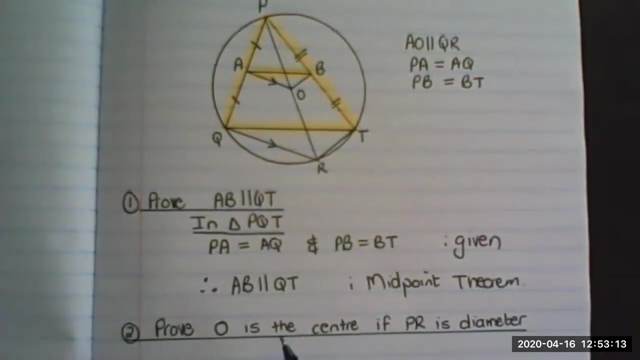 T. that information is given. therefore, a B is parallel to Q, T and the reason is midpoint theorem. and that is it. short, sweet, simple. the next question is: prove that O, that O is the center of the circle if P R is the diameter. so they say that P R is diameter and now you need to prove that that's the center of. 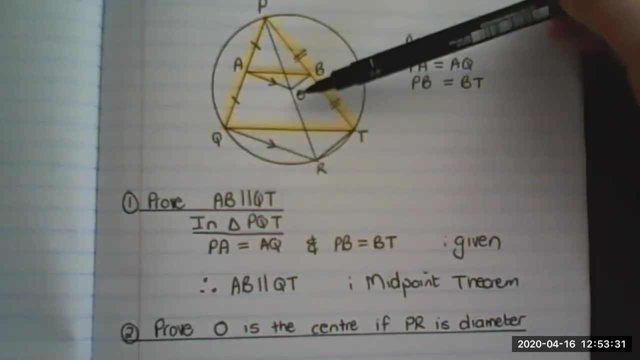 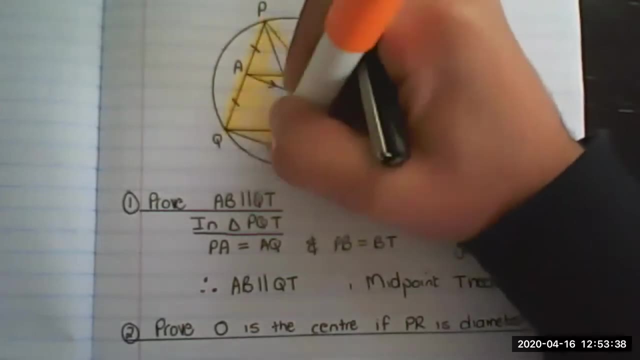 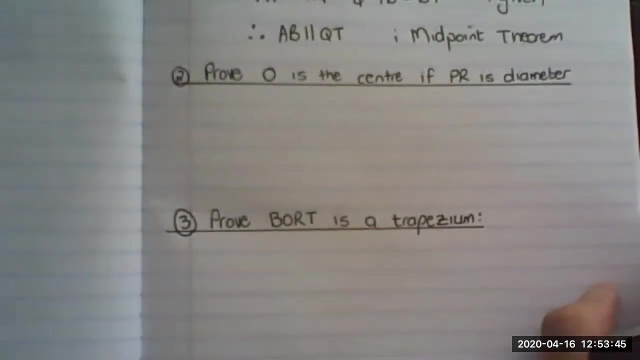 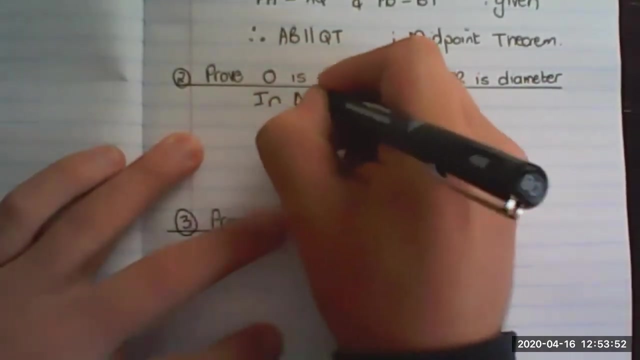 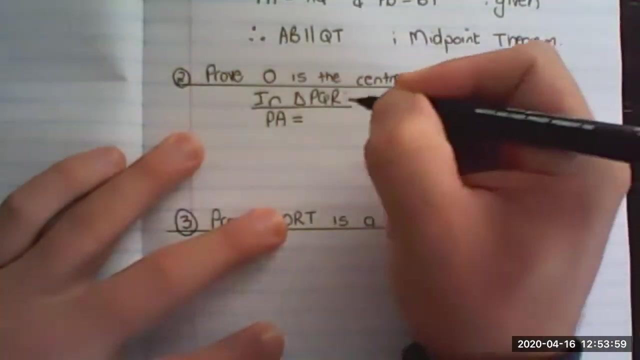 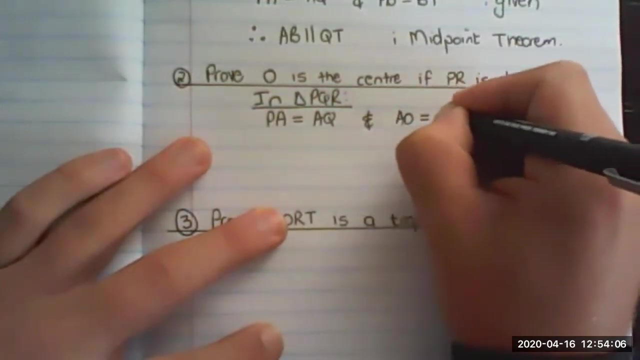 the circle. it's very simple to prove that, because we are going to look at triangle. PQ are okay, cool. let me show you how to write it. we say that in triangle, PQ are what we have is: PA is equal to a Q and a O is equal to Q R. that is given. 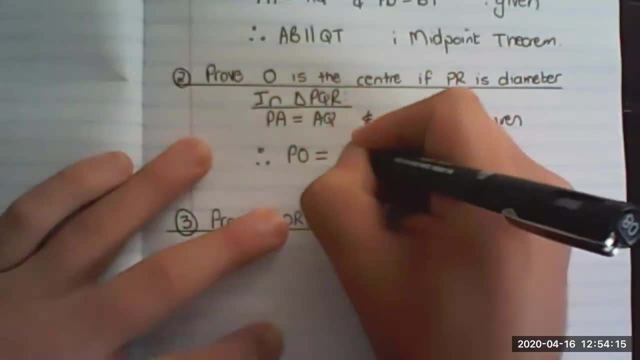 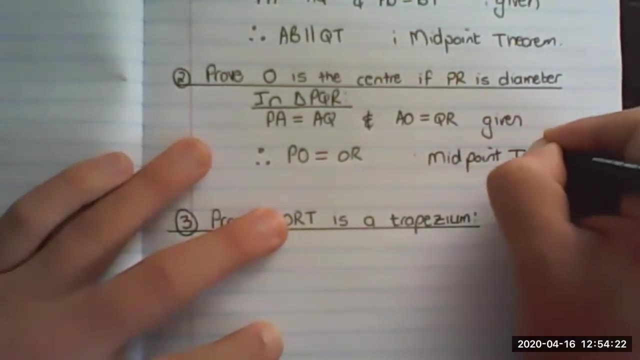 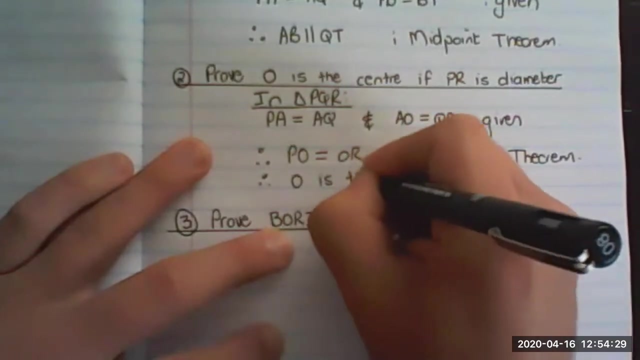 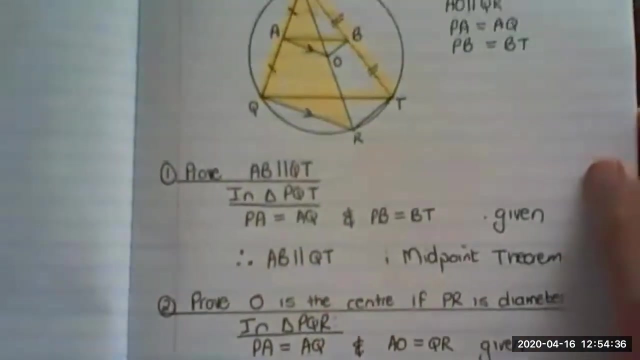 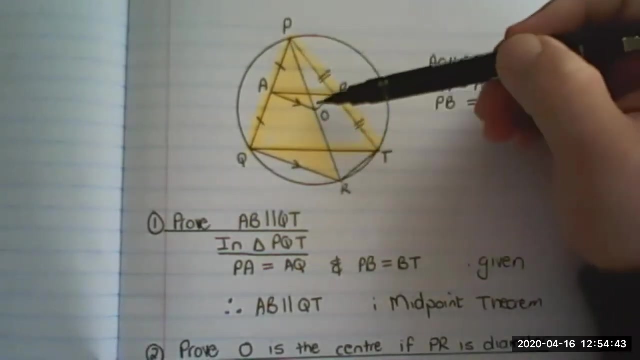 therefore P? O is equal to are the reason, or what we are using is the midpoint theorem, all right, and therefore O is the center. because that line P O equals to O, R is the diameter and because it's cut in half, that means P? O equals to aachel. siempre esta la cabeza, punto alto C cita la bruja. 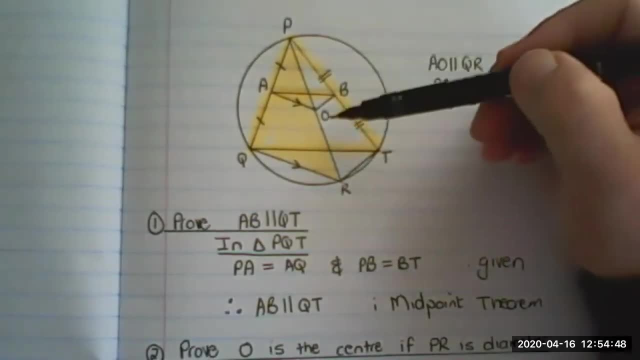 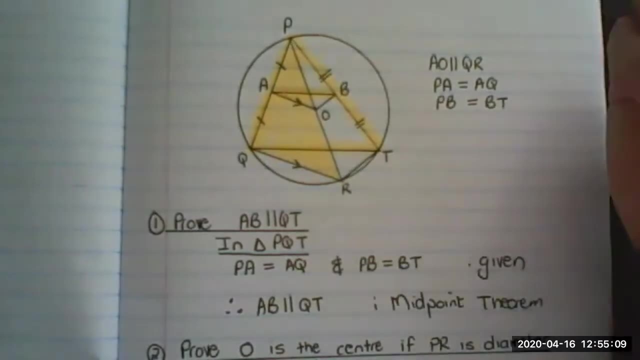 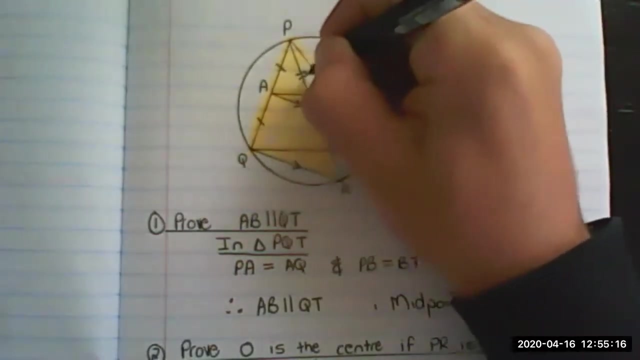 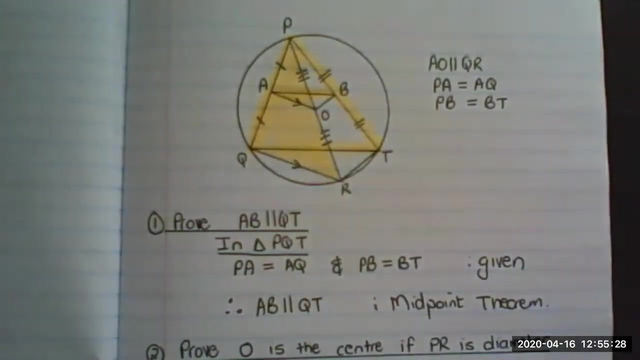 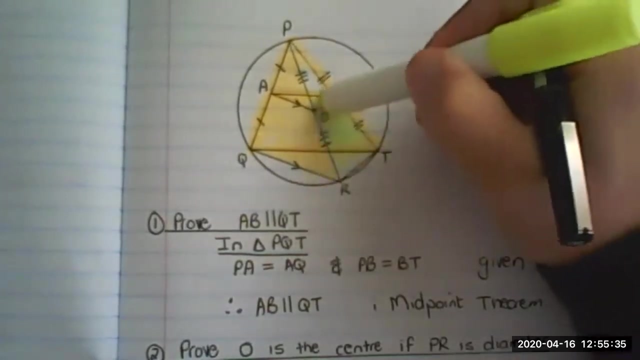 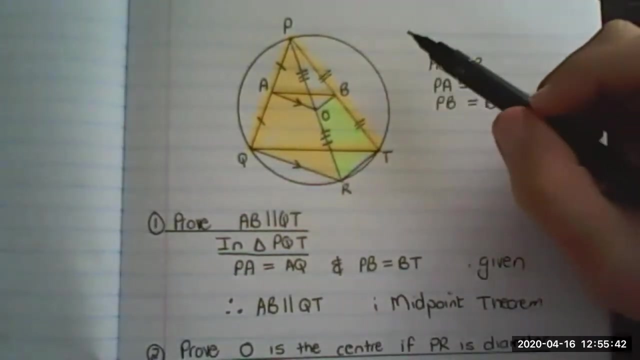 represents the radius, and or also represents the radius which makes that the center. so what we have proven now is we have added these lines equal to each other. all right. the last question is: prove that b? o r t is a trapezium. all right. what you need to prove with a trapezium is that one pair of lines or one set. 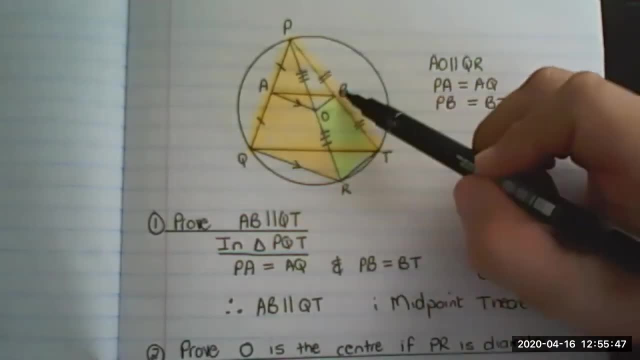 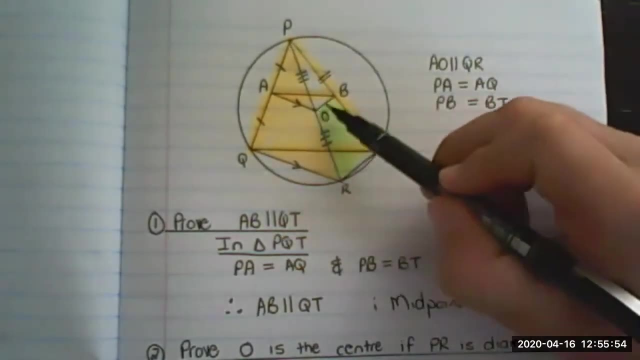 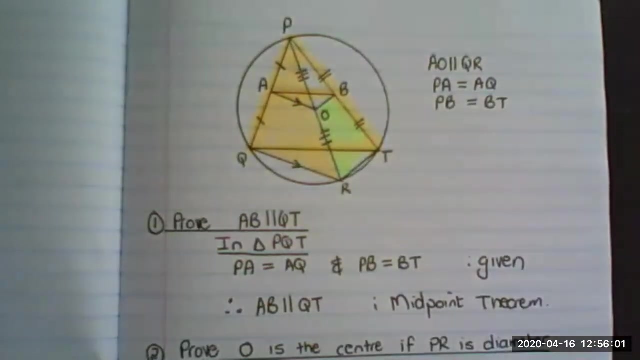 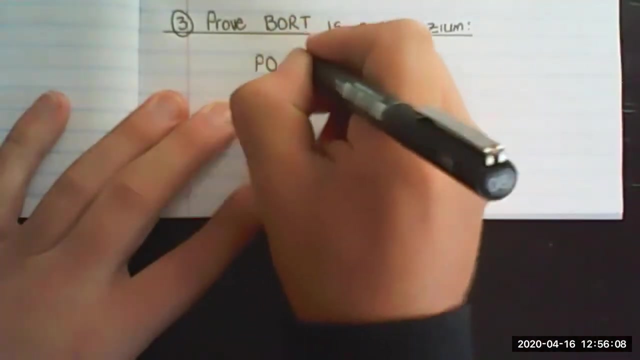 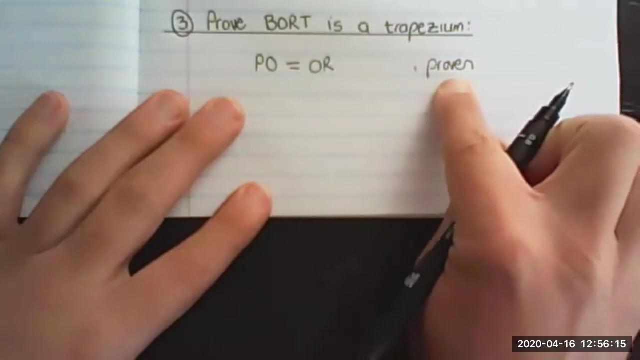 of lines are parallel. so we already have p b equal to b t and we have a p o equal to r t. therefore o b is parallel to r t, midpoint theorem- and therefore that is a parallelogram. easy way to write it is: we say: p o is equals to o r proven, it's not given. we proved it in the previous question. 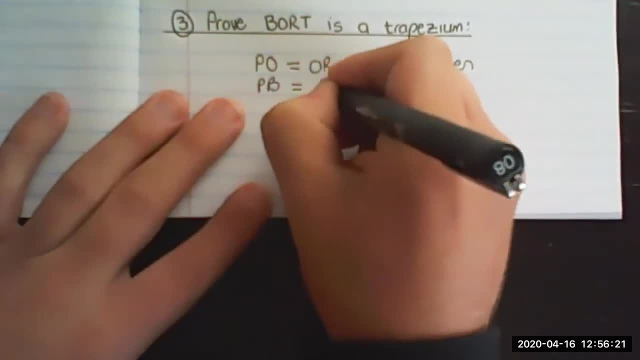 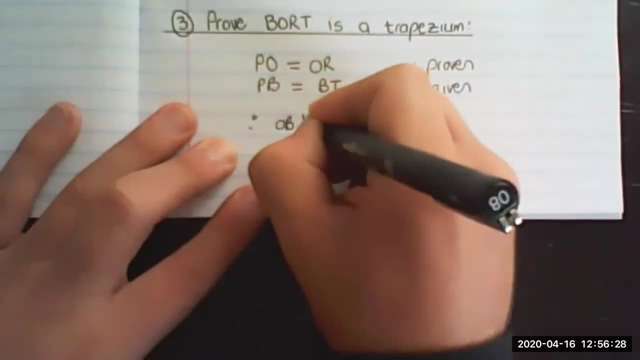 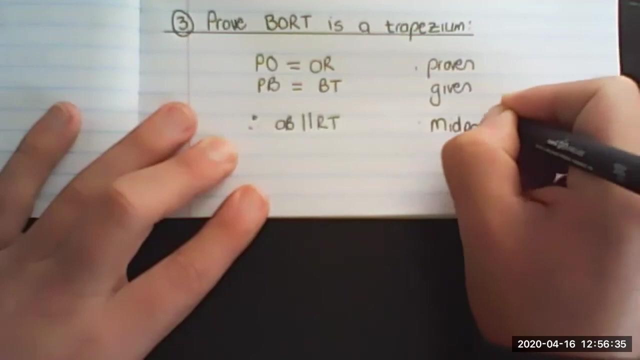 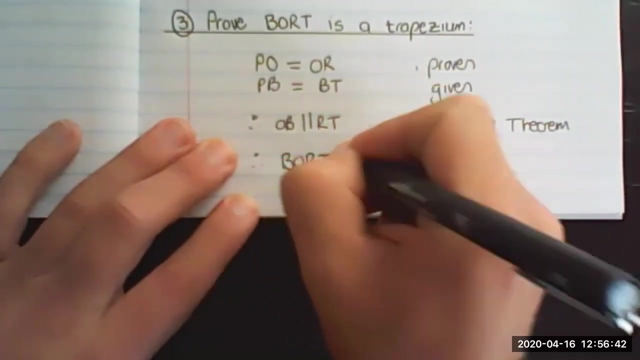 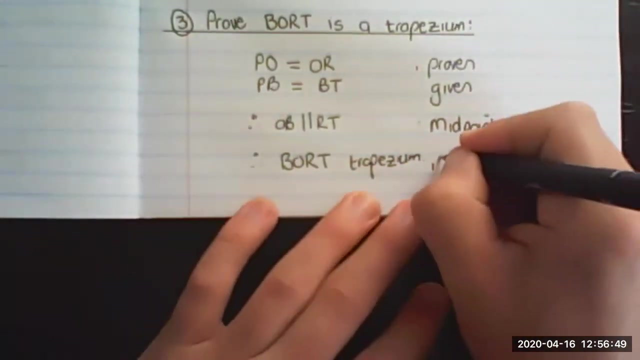 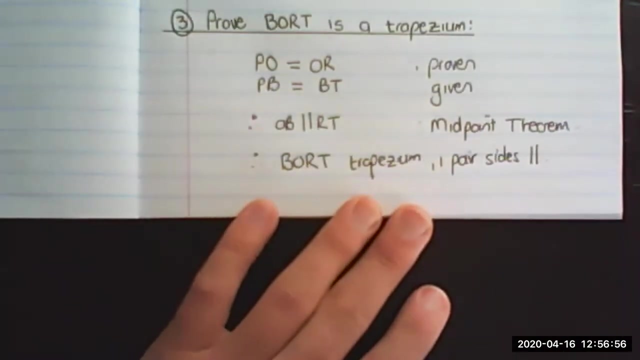 then p b is equal to b t. that information is given. therefore, o b is parallel to r t. what you've proven is the midpoint theorem. what you are using, therefore, Bo RT is a trapezium, because one pair of sides is parallel.